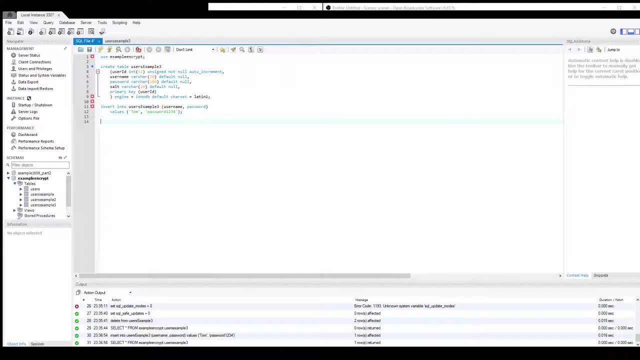 So you can do something like encryption, And MySQL actually has some built-in encryption functions that I'll show you. So this time, and you're going to call the function aes-encrypt And you'll pass in the password that you want to do, 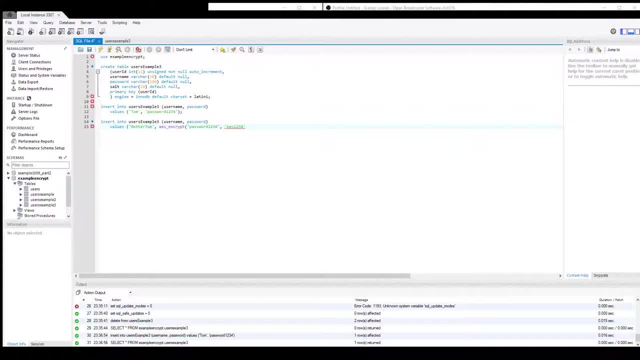 And you'll pass in a key. So what this function does is that it encrypts your password using some algorithm and it turns it into gibberish. but you can use this key to retrieve that gibberish through decryption and return it to its normal state. 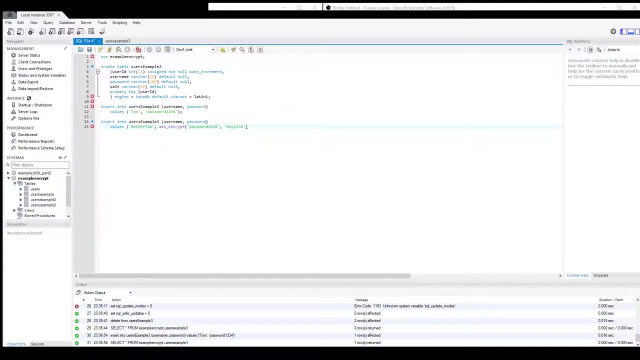 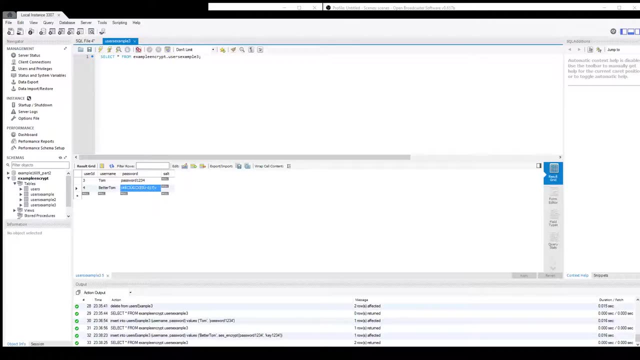 But you need to know the key. so that's the key part. So if you don't have that, you can't get the password, And this is what the password looks like right now, So you can't. no one can look at this and be like, oh, it's password 1234.. 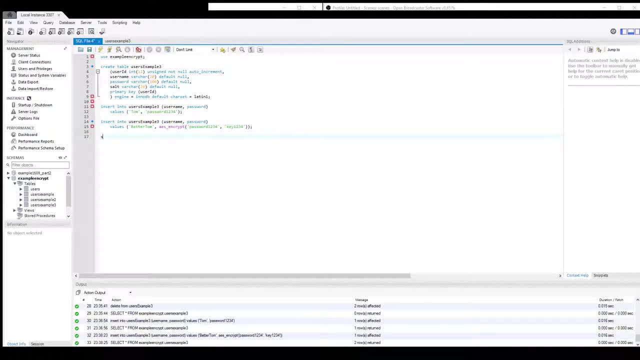 Instead, they'd have to do something like this: They'd have to decrypt it with the aes-decrypt. And they would have to do something like this: They'd have to decrypt it with the aes-decrypt. They'd have to know the key. 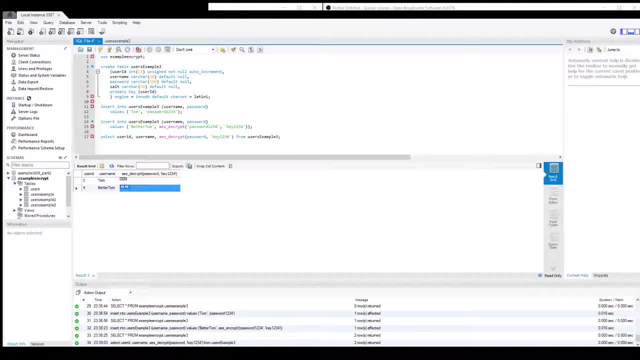 And, as you can see, it turns into blob, And I think that's because it's returning binary right now. But that's a really easy fix for me. You just cast this whole thing as a char: 100.. And voila, Password 1234, your password. 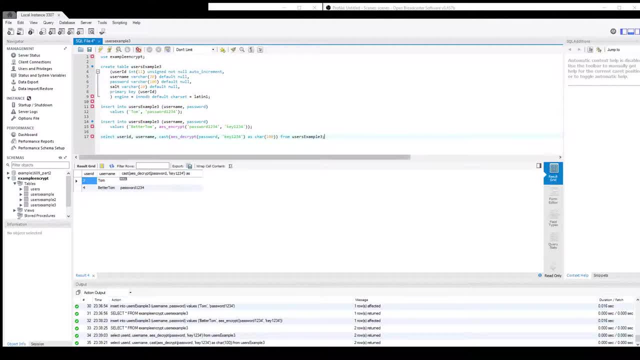 Now there is a problem that can arise from just doing something as simple as aes-decrypt. I'll show you right now. So let's say we have a person called bettertom2.. And he also chooses the same password as bettertom. 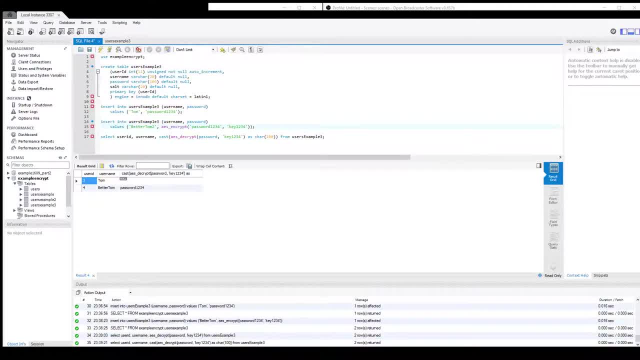 Password 1234.. That's not too unique. Anybody could easily change. There are probably hundreds of people with this password, So there's a problem that arises. Even though this password is going through this encryption, it's turning out the same. 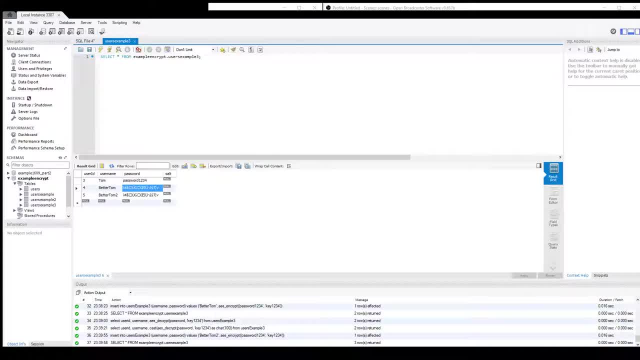 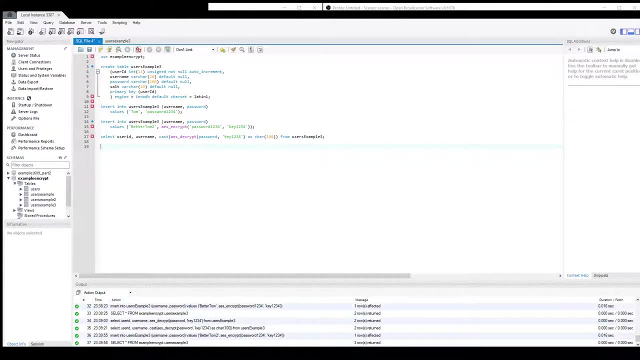 And patterns are bad. You don't want patterns because people can take advantage of these patterns. They'll be like these people have the same password And they could take advantage of that somehow. So we introduce this concept called salt, And I learned from Matt, our lab instructor today. 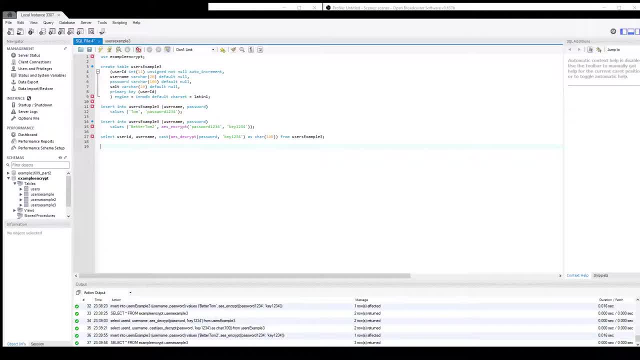 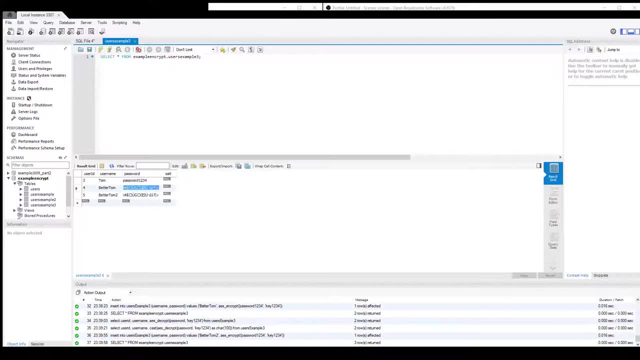 I was questioning him about salt because I was a little hazy about it, Because salt is going to stay right. You will know the salt And you'll see a decrypted password, And it seems weird to actually not encrypt salt at all, yet have the decrypted password right next to it. 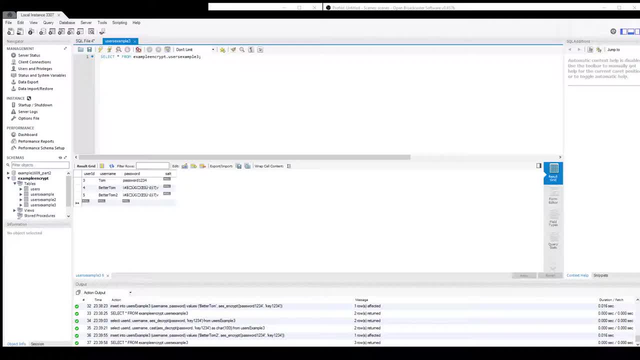 But it actually makes sense. Salt is a unique value that you concatenate with your password, So every password will have a different salt right next to it And when you push it through that AES encrypt it's going to turn your password into something different. 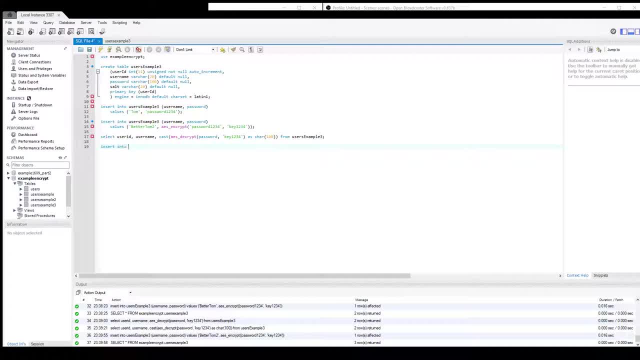 And I'll show you that right now. So insert: This time we're going to add salt, So we're going to send in the concatenation of password 1234 and your salt And you're going to send in the same key as usual. 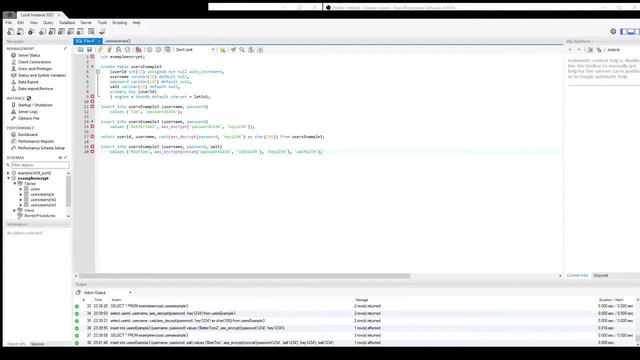 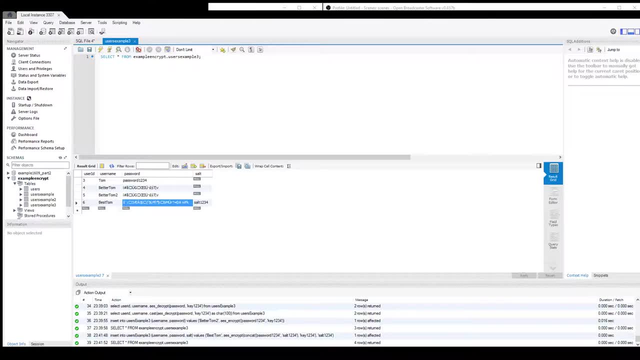 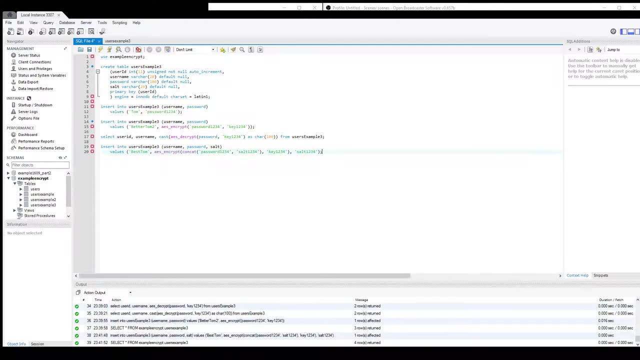 And what you'll notice is that your password- even though it's password 1234, is completely different than these. So when you do something like this, When you have the same password- And let's say, there's a best time too- 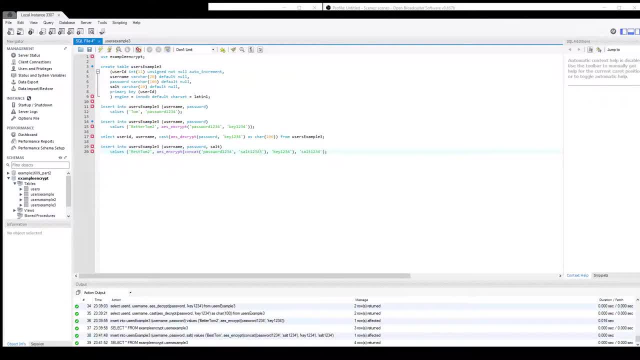 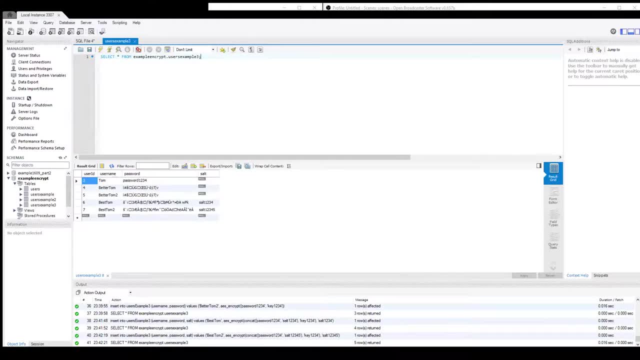 You have a different salt And this way They look different. So that's something that you can actually add to make your encryption a lot stronger, And it seems weird to include it here, but you actually need it to decrypt it And yeah. 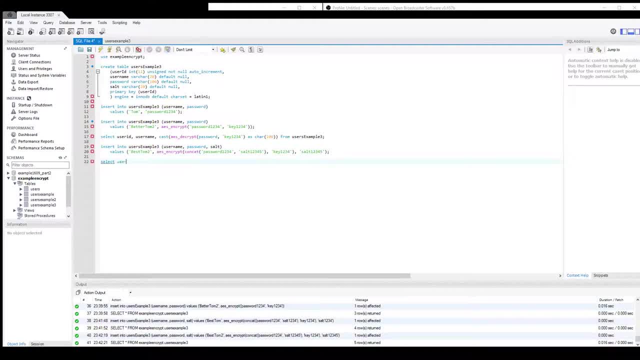 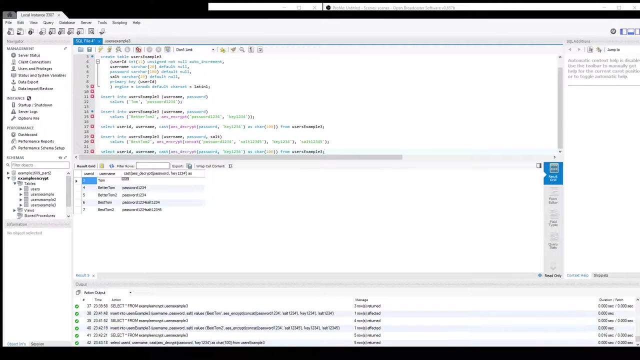 So I'll show you how to decrypt it. So do this. I'll do that later. So aes: Decrypt Password Key 1234.. I'll cast that As a char: 100.. Done, So, as you'll see, 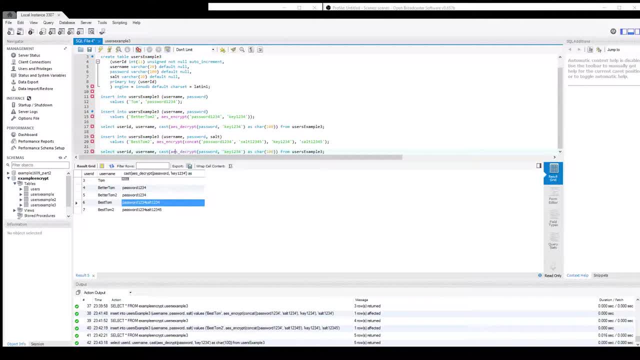 You can see the salt is concatenated from it. So all you have to do is remove from this string your salt And replace it. So replace My bad, Replace your salt with nothing, And I forgot to do that earlier. So once you replace your salt with nothing, 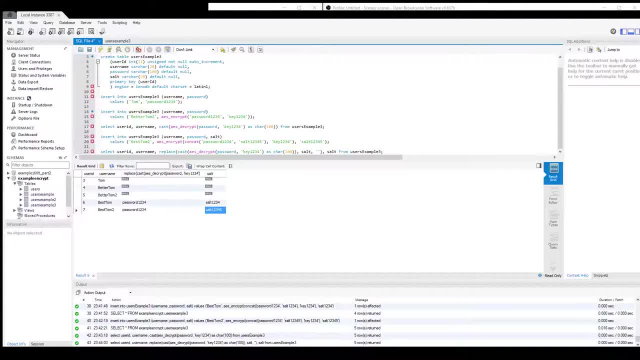 You'll get your password Done. So, as you can see, This is just barely scratching the surface, Barely scratching the surface of encryption. People can make their own encryption algorithms that might be way better than these. They can come up with ways of generating the salt. 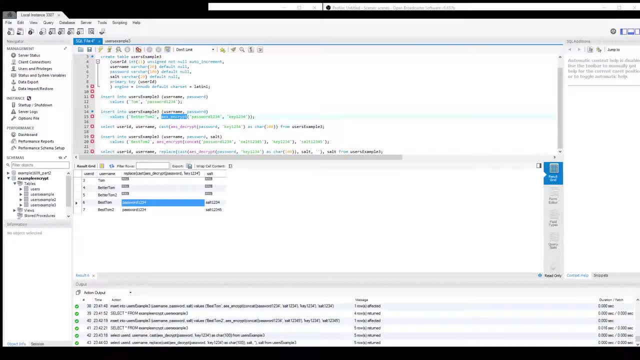 And generating the keys Bunch of hash functions that are involved. And yeah, It's just a topic that really expands Because as people get As encryption algorithms get better, People get better, So it always has to be improving.